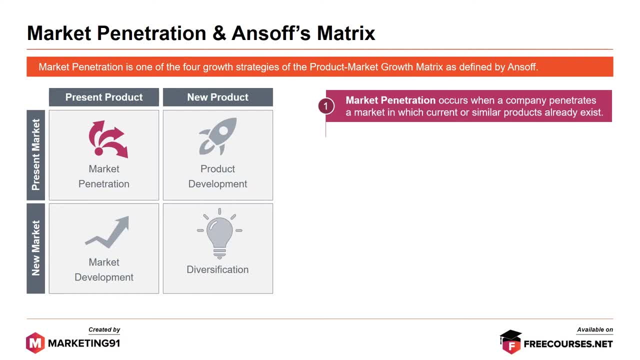 Market Penetration occurs when a company penetrates a market in which current or similar products already exist. A way to achieve this is by first, gaining competitors' customers, and that is part of their market share. Next, attracting non-users of the product. And third, 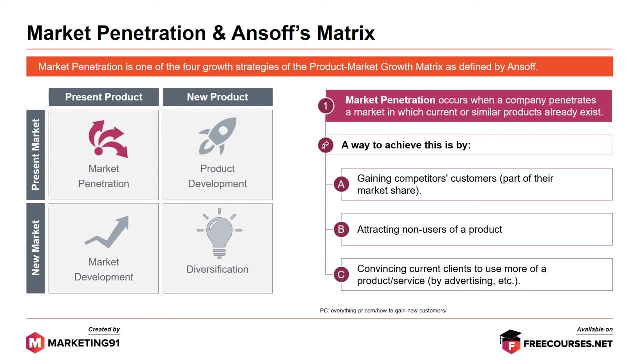 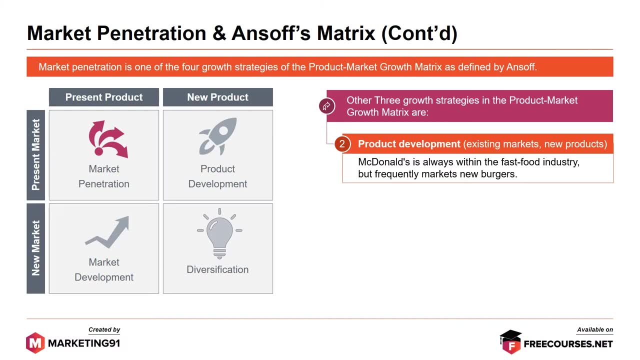 convincing current clients to use more of a product or service by advertising. The other three growth strategies in the Product Growth Matrix are: second, product development, that is, existing market and new products. Example here is McDonald's. Third, market development, as in a new market with existing products, which Apple does by introducing. 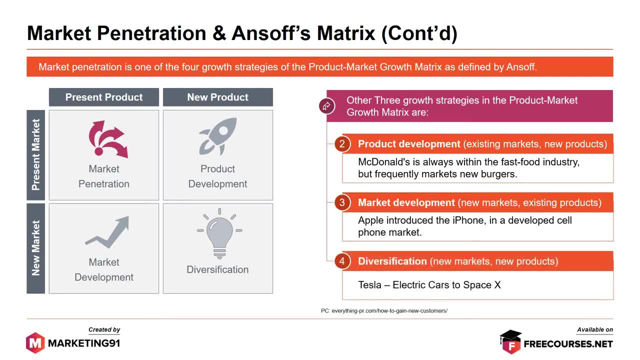 the iPhone in an already developed cell phone market. And finally, diversification- The example in this case is Tesla: The new market with existing products, which Apple does by introducing the iPhone in an already developed cell phone market. And finally, diversification. The example in this case is Tesla, The. 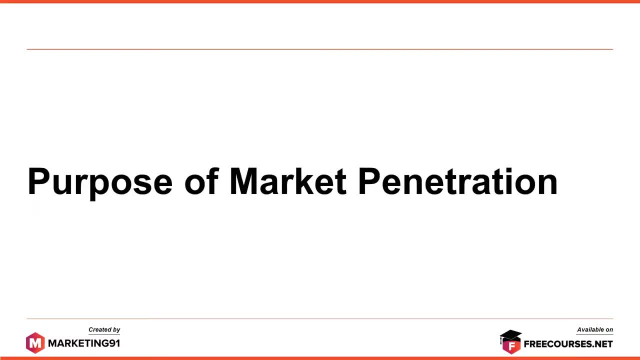 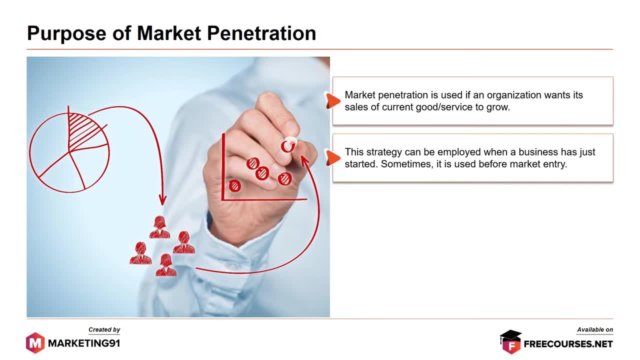 to grow. The strategy can be employed when a business has just started. sometimes it is used before market entry. In a high market penetration, a Biz can show that it has a presence in the market. It can show the market size for the goods or service. 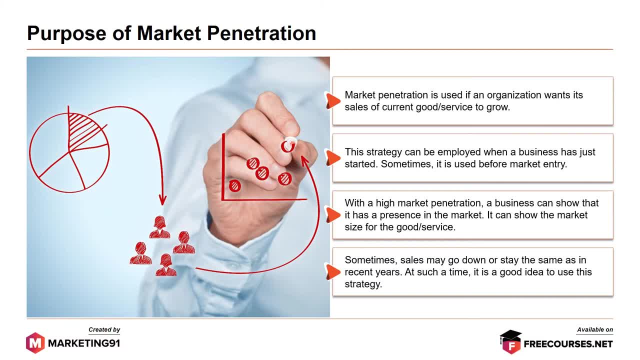 Sometimes sales may go down or stay the same as in recent years. As such a time, it is a good idea to head to and use this strategy for scrutinization sontGuide by Microsoft. New York is afforded for the product in, say the amount needed. 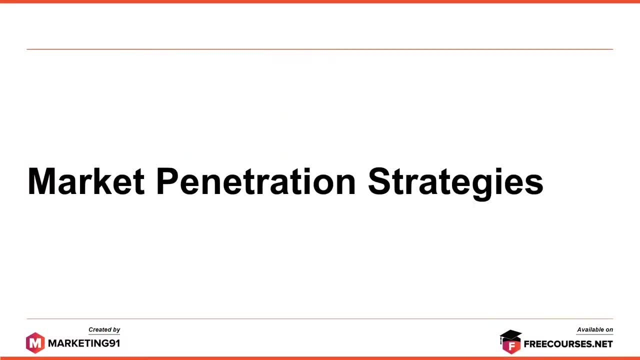 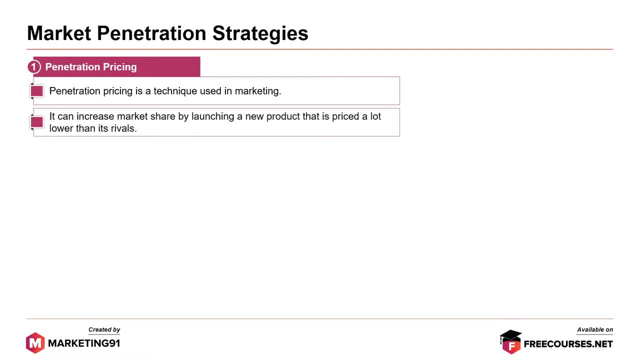 Crumba undies and provides for the beginning of the long run, So I missed existing products. Next, let's look at market penetration strategies, The first being penetration pricing. Penetration pricing is a technique used in marketing. It can increase market share by launching a new product that is priced at lower level than its rivals. 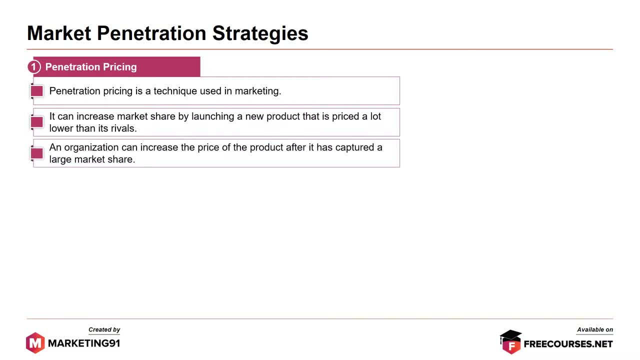 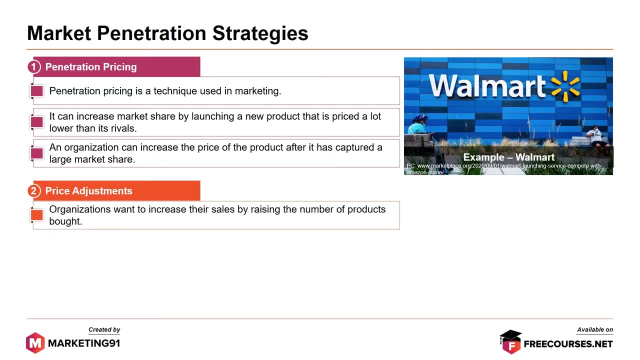 An organization can increase the price of a product after it has captured a larger market share. Example: Walmart. The next strategy: price adjustments. Organizations want to increase their sales by raising the number of products bought. They do this by lowering the prices below their rivals for customers. 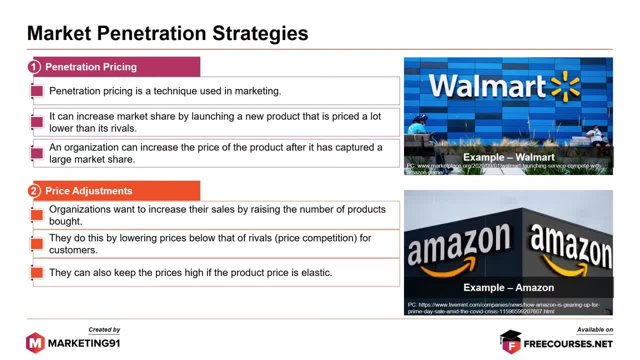 They can also keep the prices high if the product price is elastic. The best example in this case is Amazon. The price of an average product shifts every 10 minutes, which means Amazon changes product prices about 2.5 million times daily. The third strategy: increased promotion. 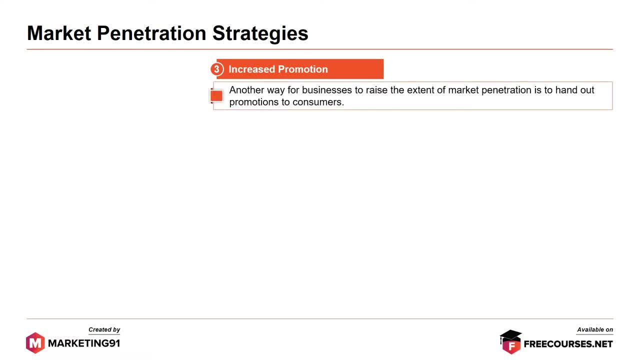 Another way for business to raise the extent of market penetration is to hand out promotions to customers. The strategy of promotion relates to pricing. It increases the brand awareness of the product. It raises profit And captures a higher market share. The best example in this case is Vivo, a Chinese smartphone brand. 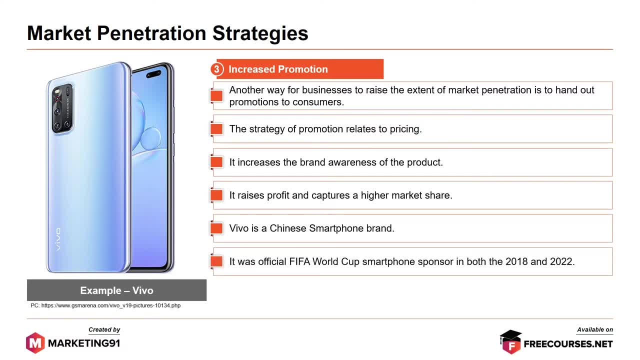 It was the official FIFA World Cup smartphone sponsor in 2018 and for the upcoming World Cup in 2022.. Financial Times claims that the agreement is worth 400 million euros. Next, increased distribution channels. A distribution channel connects an intermediary to a business. 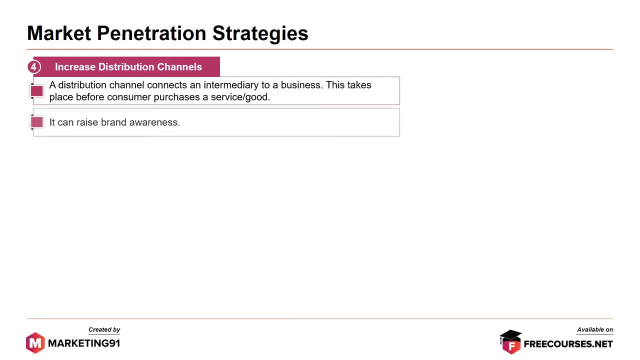 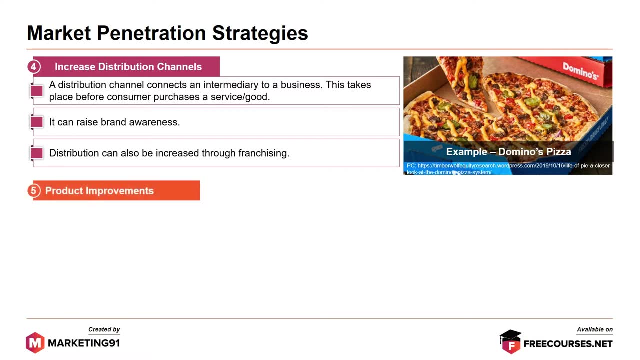 This takes place before the consumer purchases a service of good. It can also raise brand awareness. Distribution can also be increased to franchising. The best example in this case is Domino's Pizza. The company's market share in India is believed to be increasing because it expanded franchises. 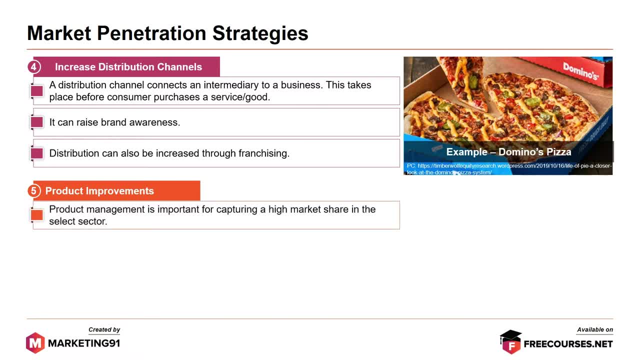 Next, product improvements. Product management is important for capturing a high market share in the select sector. Organizations can beat rival products by bettering the quality of their own. They can also meet customers' needs and attract them. This leads to a higher sales volume. 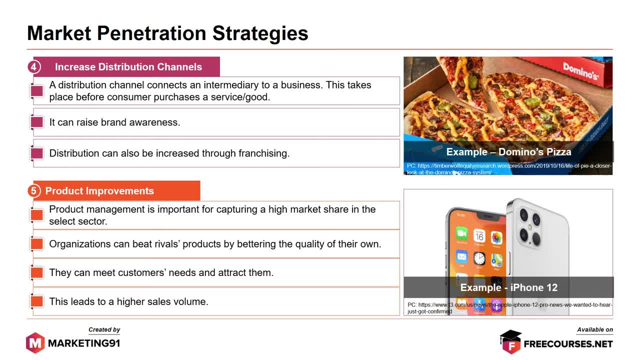 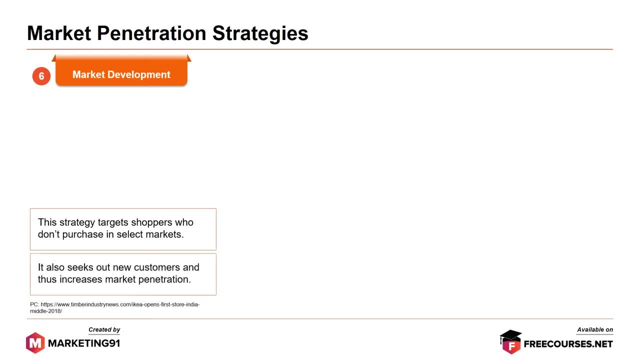 The best example in this case is Apple's iPhone 12 sales. The next one: market development. This strategy targets shoppers who don't purchase. It also seeks out new customers and thus increases market penetration. Example: IKEA. On December 18, 2020, IKEA set up its second store in India. 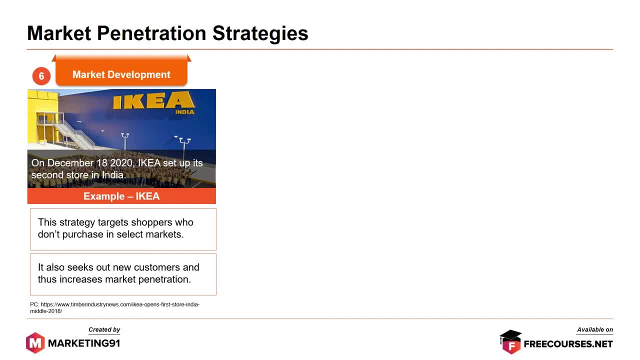 IKEA plans to invest INR 6,000 crores over a decade in India. By 2020, it plans to cater to 25 million people in the state of Maharashtra in India. Seventh, develop strategic alliance. Retail brands can create and strengthen partnerships by signing co-branding deals or mergers. 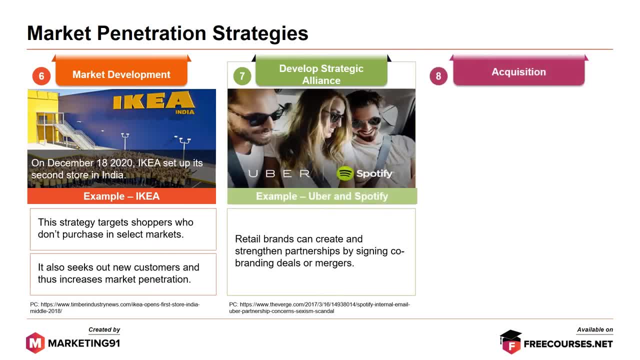 The best example in this case is Uber and Spotify. And finally, advertising. Buying a store is similar to state-of-the-art acquisition. Acquiring a new rises in the same industry is the same as purchasing the business' customer base. The market share of the business is thus also captured with it. 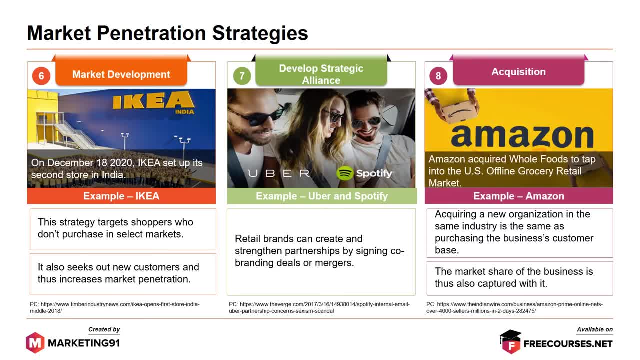 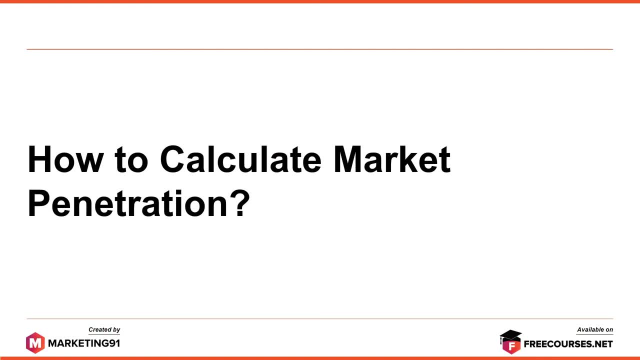 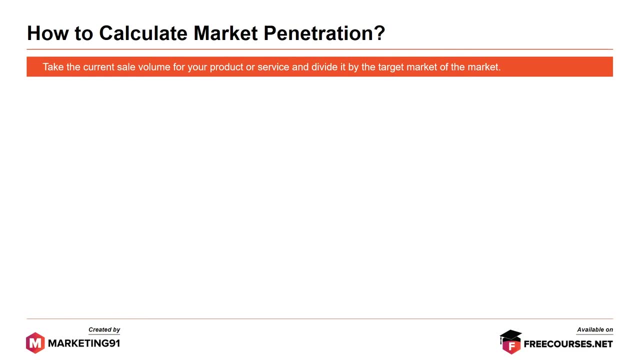 The best example: Amazon's acquisition of Whole Foods to tap into the US Offline Grocery retail market. Next, how to calculate market penetration: Take the current sale volume for a product or service and divide it by Target Market of the market Formula – number of customers divided by target market size and 200. 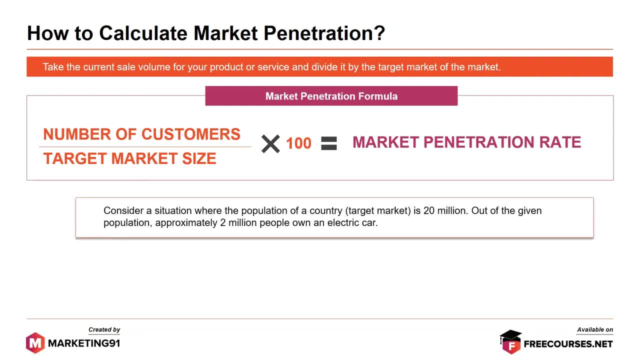 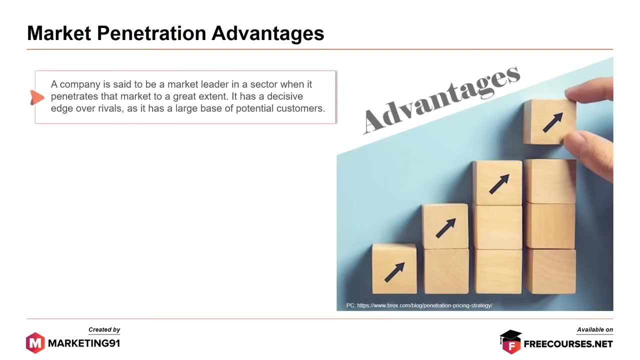 gives you the market penetration measuring rate. Consider a situation where the population of a country is 20 million. out of the given population, approximately 2 million people own an electric car. Then the market penetration of electric car will be 10%. Moving on to market penetration advantages, A company is said to be a. 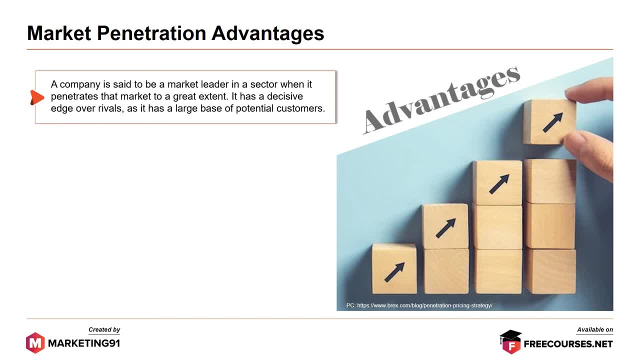 market leader in a sector. when it penetrates the market to a great extent, It has a decisive edge over rivals and it has a large base of potential customers. A market leader can strike out better legal suppliers. This is because bulk deal orders can now be placed thanks to a larger market share, and 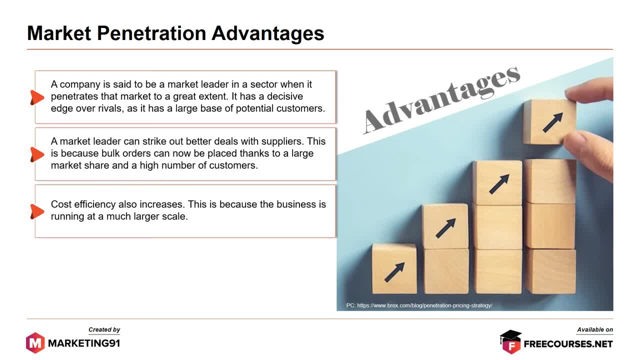 high number of customers. Cost efficiency also increases. This is because the business is running at a much larger scale. In retail, a market leader gets better positioning and larger shelf space in comparison to competitors. This is because their good services enjoy much higher popularity among consumers. 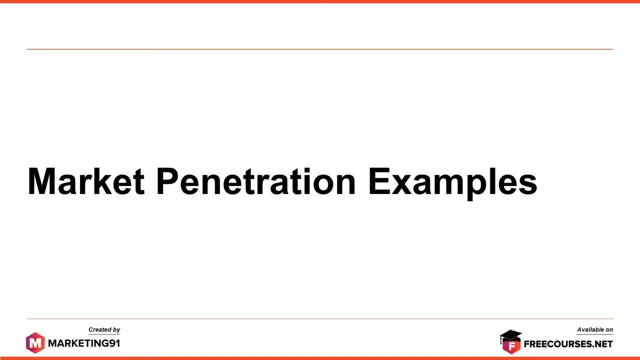 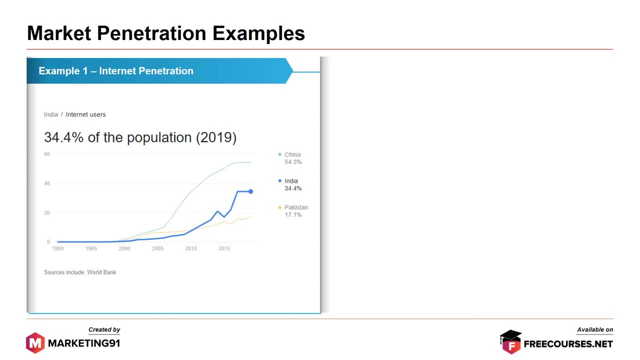 Moving on to some examples of market penetration, The first being the internet penetration. India's internet penetration is 34.4% of the total population, whereas China's is 54.3% and Pakistan's 17.1%. Next, global electric. 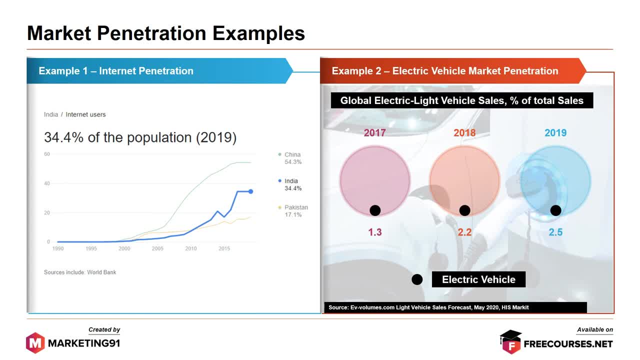 vehicle market penetration: In 2017 it was 1.3%, which moved up to 2.2% in 2018 and in 2019 the global electric light vehicle sales penetration of the total automobile market was 2.5%. Example third: the smartphone user. 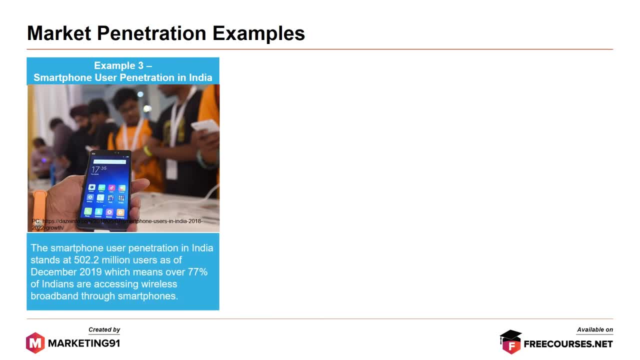 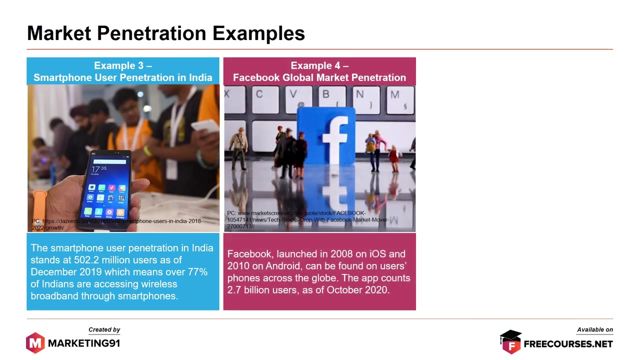 penetration in India. The smartphone user penetration in India stands at about 502.2 million users as of December 2019, which means a 77.0% of Indians are accessing wireless broadband through smartphones. Next, Facebook's global market penetration. Facebook launched in 2008 on iOS and 2010. 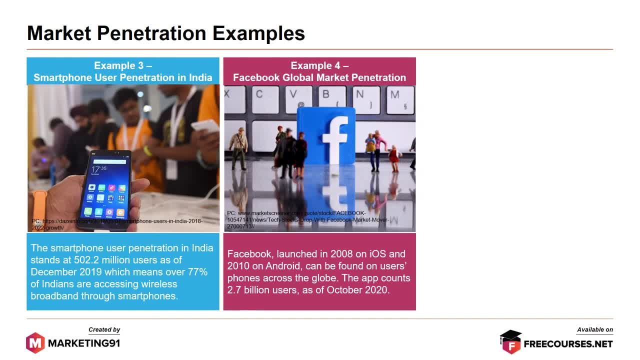 on Android and can be found in users phones across the globe. The app counts 2.7 million users as of October 2020.. India is the single biggest market for Facebook, with 269 million users as of 2019.. And the final example of Instagram's market penetration. 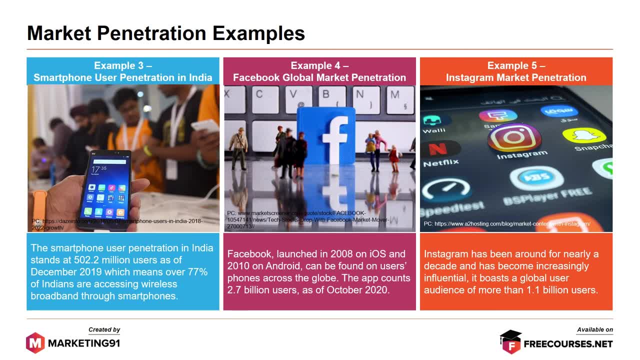 Instagram has been around for nearly a decade and has become increasingly influential: It boasts a global user audience that marks an income increase of 5.1% in 2019.. influential: It boasts a global user audience of more than 1.1 billion users.